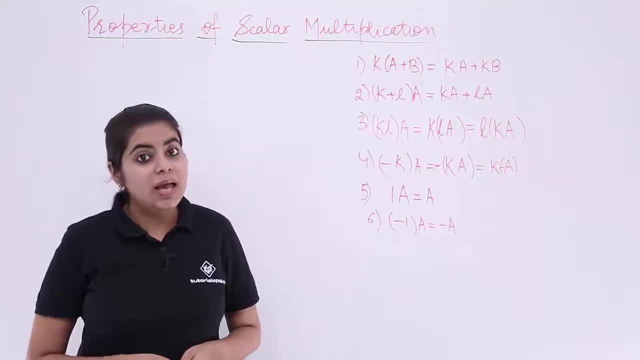 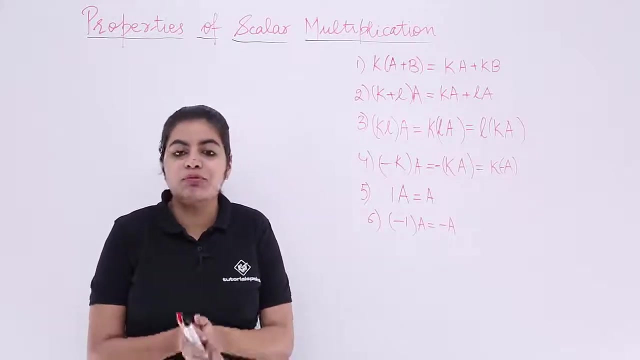 In this video, let's see another topic based on properties in mattresses, which is known as properties of scalar multiplication. As you can see here, I have enlisted nearly six properties on the board, and these six properties are important for learning point of view and understanding and not from proof point of view, So we will not be seeing the proof. 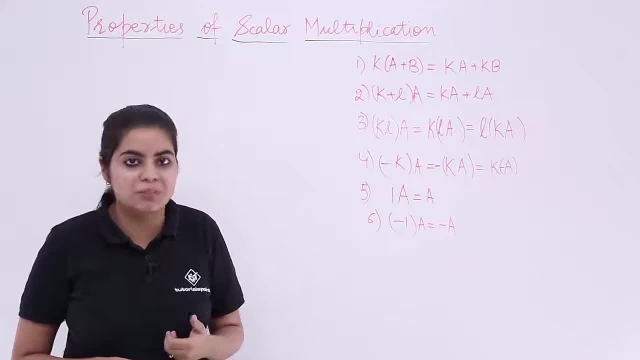 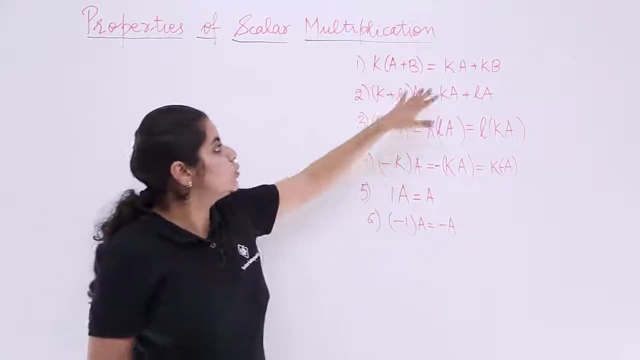 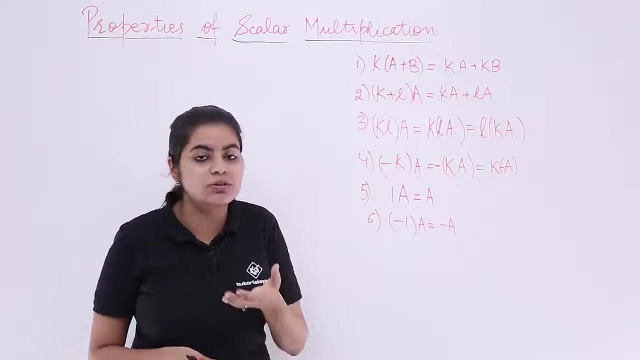 rather, we will be seeing these properties with the help of few examples. So what is the first property? The first property is k into a plus b- in the brackets is equal to k a plus k b. I want to illustrate that in these videos we will be taking up few scalar quantities, As you can see. 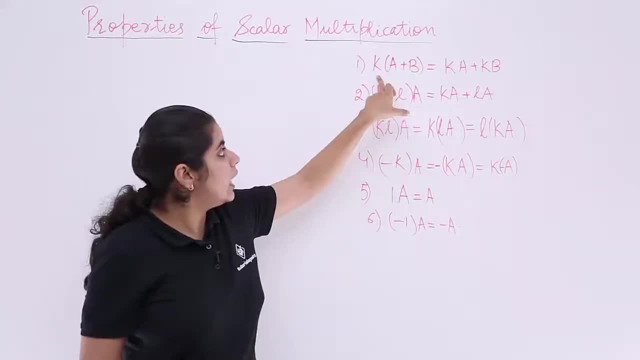 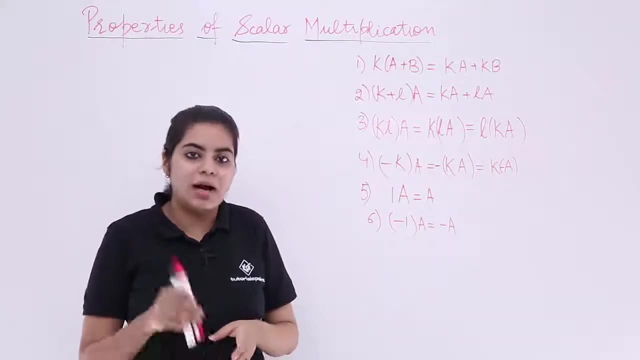 the heading was what Scalar multiplication- That means k, which is used- is a scalar quantity. You will be finding here l, l is also a scalar quantity and there are few mattresses which are available in this video which are a- b that we will be taking into consideration. Now moving 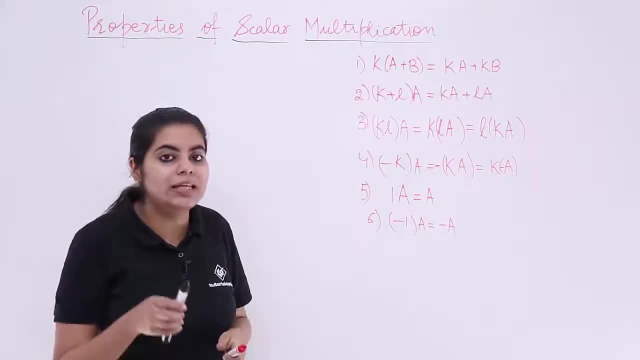 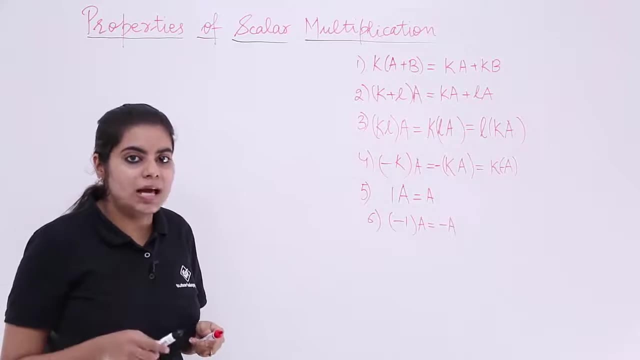 on to the next topic. let's see how to calculate the property of scalar multiplication. So the first property, k into a plus b, is equal to k a plus a b. Now let's see k a plus k b is there. We will be seeing it with the help of an example and we will prove it accordingly. only The first. 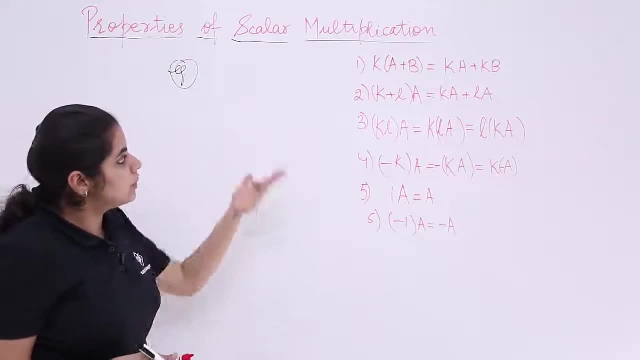 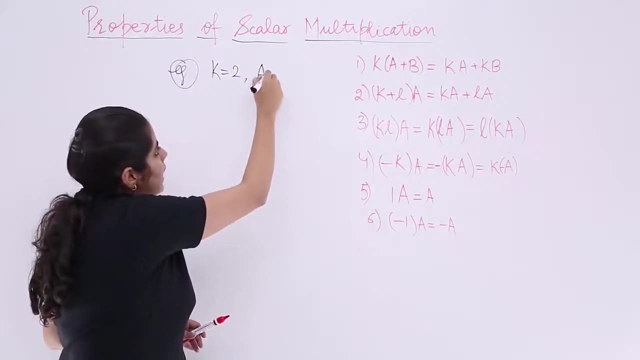 proof with the help of the first example. Suppose I have two mattresses and the value of k is given to me as 2.. k is a scalar. It is given to me as 2.. I have matrix a given to me as, say, 5 and 9. 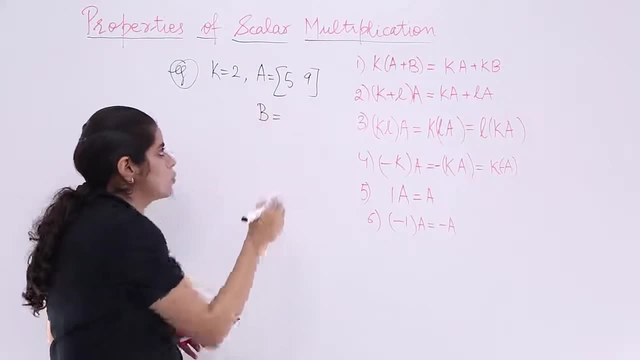 which is a row matrix. I am taking simple example. I am taking simple example. I am taking simple example just to prove the basic things right. I have a matrix b which is say, 9 and 5.. Now, what am I? 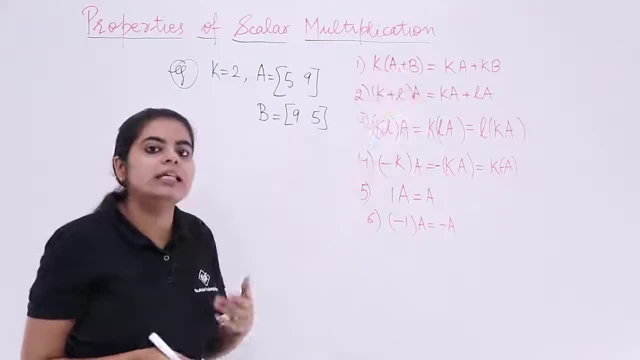 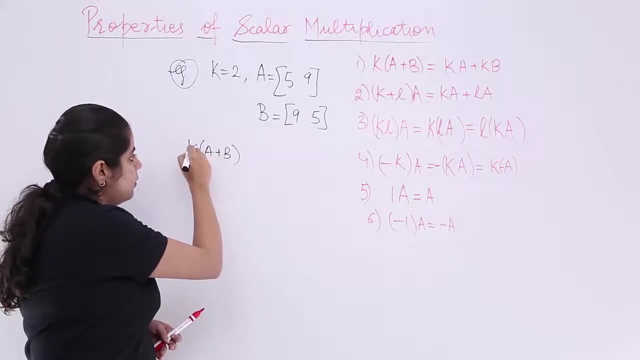 supposed to do. We are basically proving this with the help of an example, and this is the illustration as well. The left hand side is what It is: k into a plus b, as you can see right. So it is k into a. 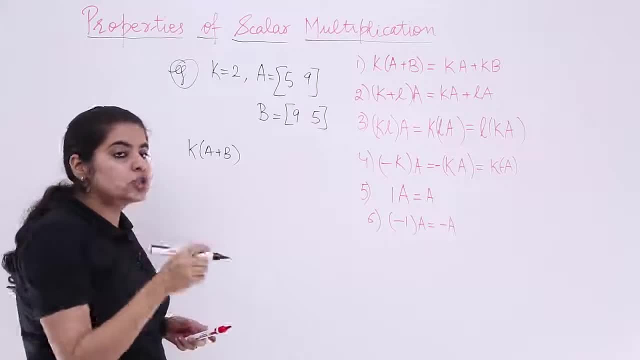 plus b. What is the value of k? k is basically 2.. 2 will remain there as it is. What about a plus b? a plus b means you have to add the 2 to a plus b. So you have to add the 2 to a plus b. So. 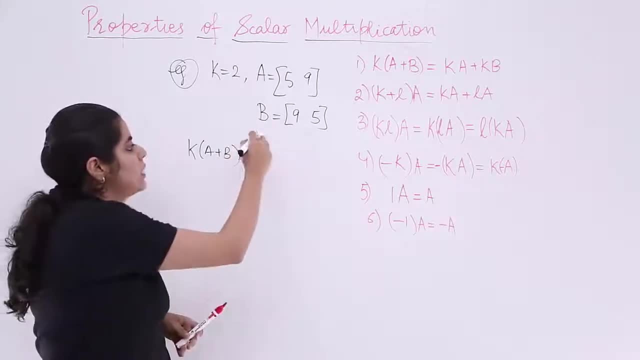 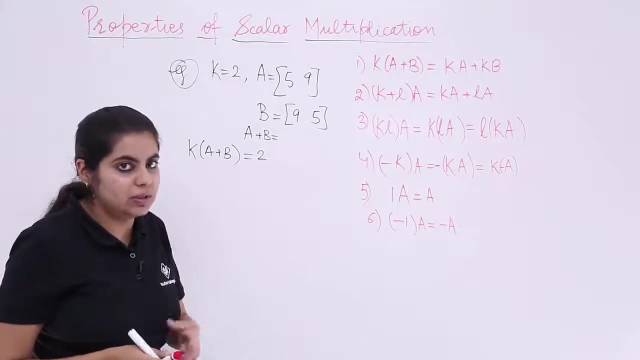 you have to add the 2 matrices a and b. a and b. What is a plus b? First? we will be writing here only. So a plus b is a new matrix with the same order as a and b. What was the order here? It was: 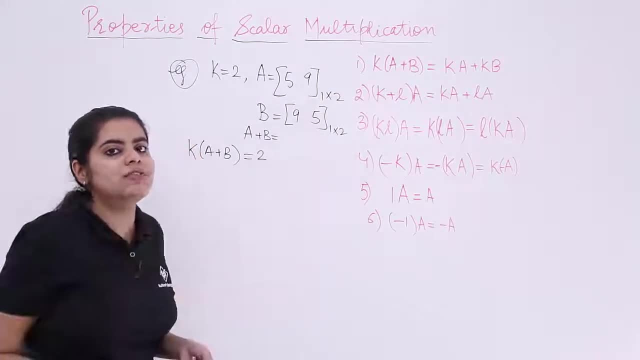 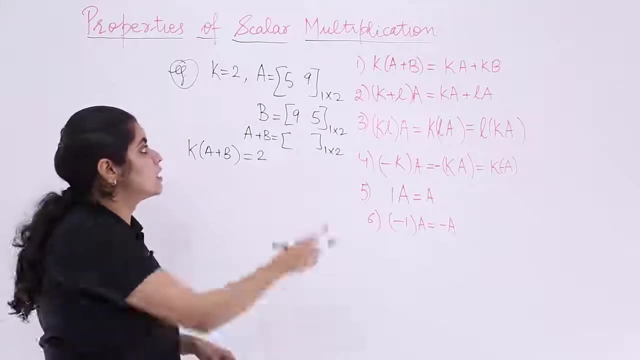 1 row and 2 columns. 1 row and 2 columns. New matrix also has how many rows? 1 row and 2 columns. a plus b means addition of both these matrices. What is 5 plus 9?? It is 14.. What is 9 plus 5?? 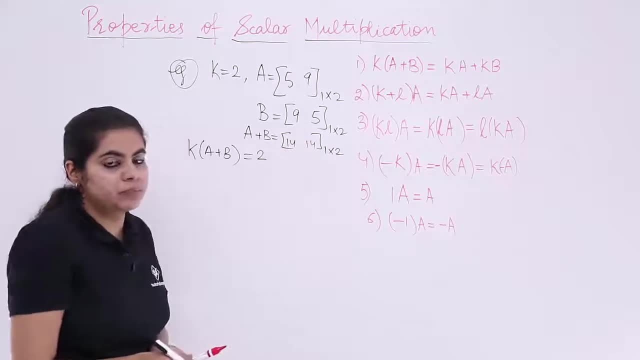 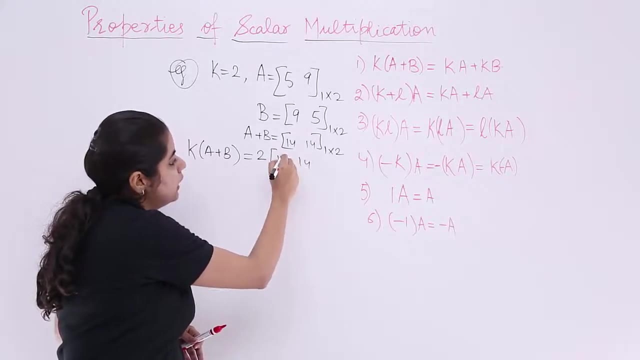 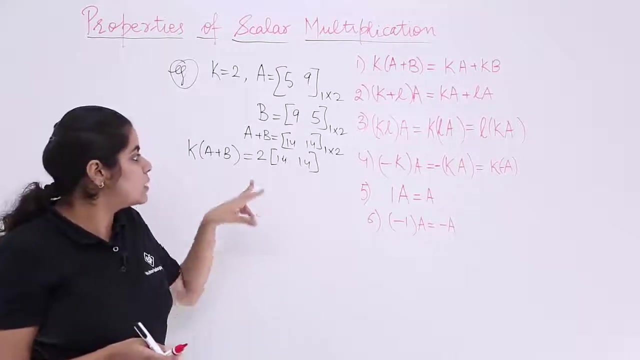 Again 14.. So it is 14 here, 14 here. Put the value of a plus b in this equation: 2 into a plus b means 2 into 14 and 14 which is inside. Now you know that the matrix multiplication in the case of scalars goes the manner that 2 will. 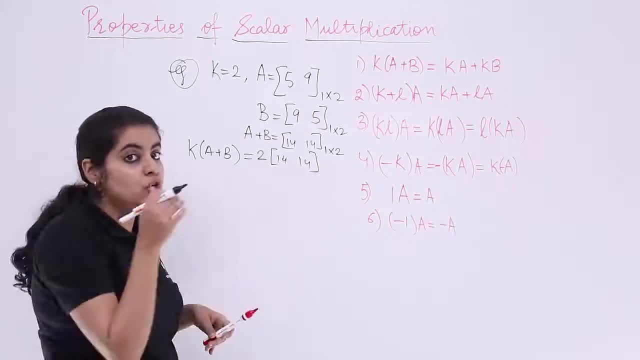 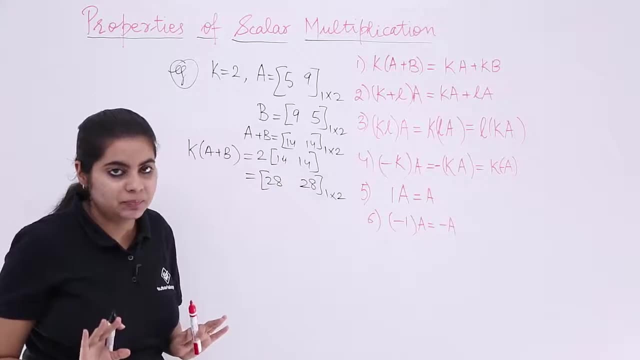 be multiplied with 14 also, and this 14 also. So what answer do I get? I get 28.. 28 as a 1 by 2 row matrix. In the case of k into a plus b, it is 14.. So what is the value of k? k into a plus b. So 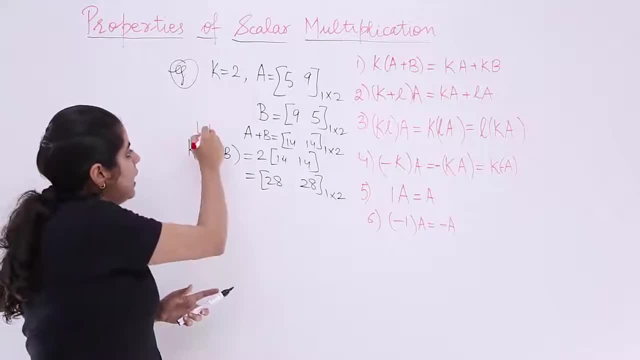 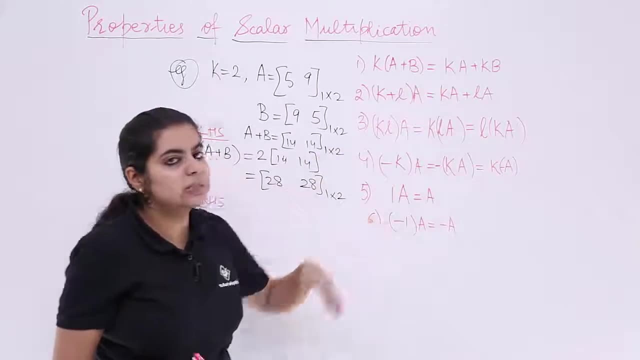 what is the value of k k into a plus b? Now, this was the left hand side. I write here LHS of the proof. Let's go with the right hand side and if the answer is same, we can prove the first property. 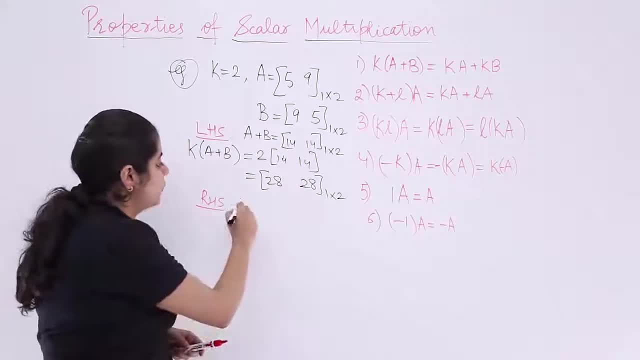 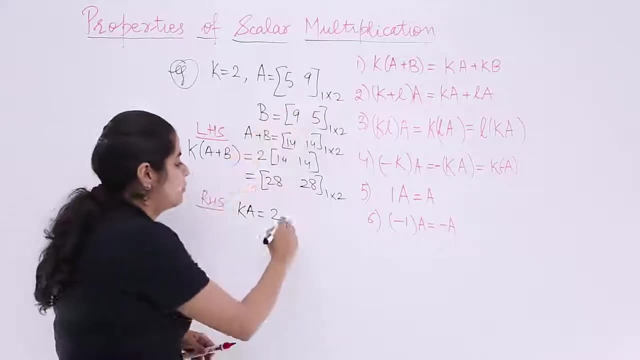 What is the right hand side? It is ka. What is ka? Ka means that you need to multiply 2.. 2 is the scalar with a. What was the? a matrix 5, 9.. Now, what happens when we multiply it in this manner? 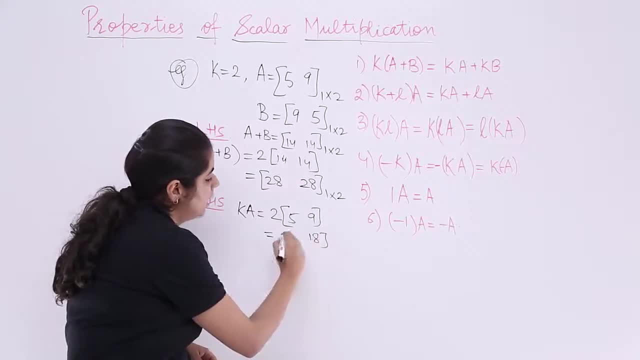 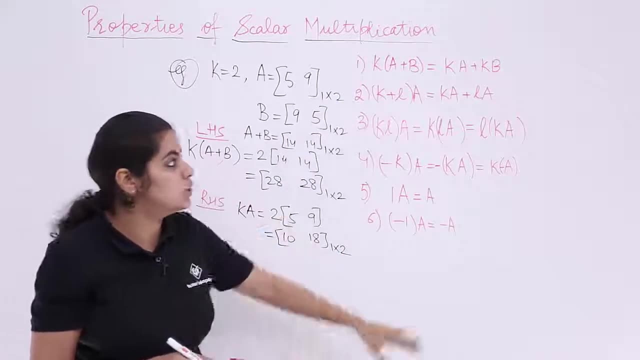 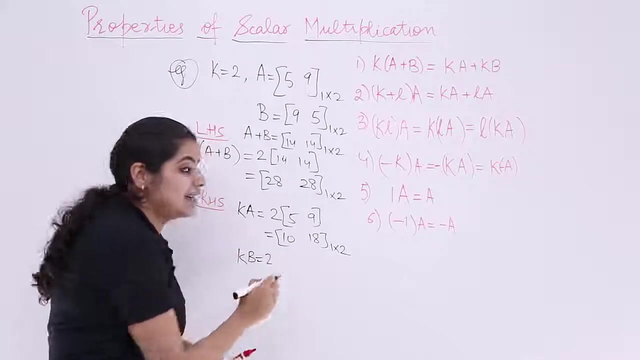 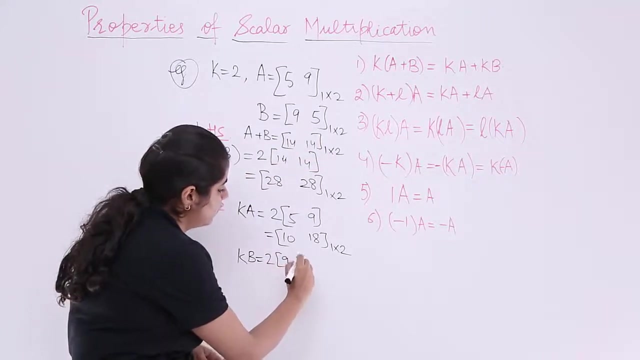 2, 5 becomes 10.. 2, 9 becomes 18.. We get a matrix as 10, 18 of the order 1 by 2.. This is done for ka. Similarly, you need to go about doing for kb. What is kb? kb means 2 multiplied by the matrix b. What is matrix b? Matrix b we took as 9, 5.. You can see there. So it is 9, 5.. Now 2, 9 is 18.. 2, 5 is 10.. So it is 18 and 10.. 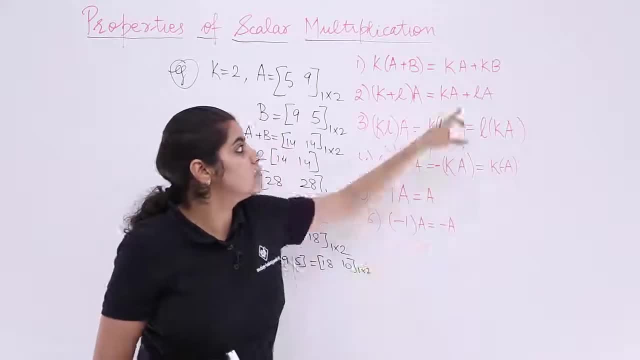 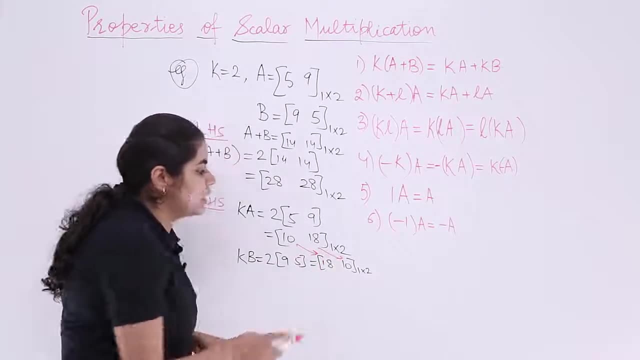 What we were supposed to do now. We are supposed to basically add these. You see, here it is a plus sign. So add these 10 plus 18.. Add the first elements, Add the second elements. 10 plus 18 is 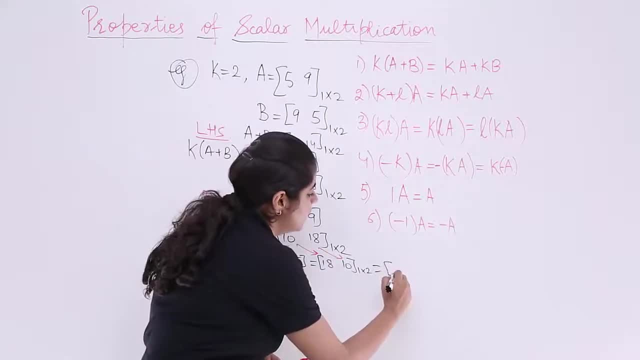 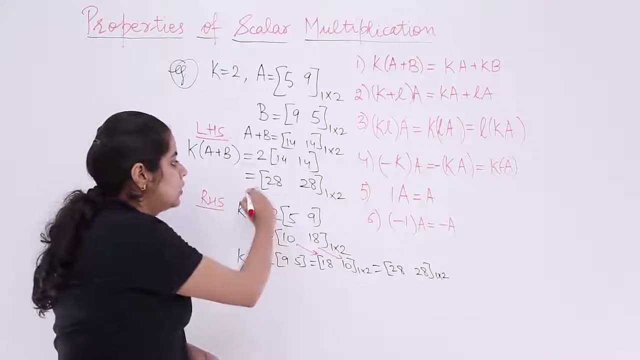 28.. Here also, 18 plus 10 is 28.. So basically I get a new matrix which is 28 and 28, and it is a 1 by 2 matrix. Now you see here, Here also it is 28 and 28.. Here also it is 28 and 28.. That means what? 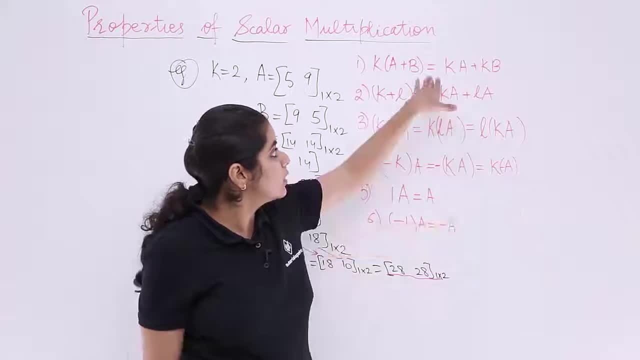 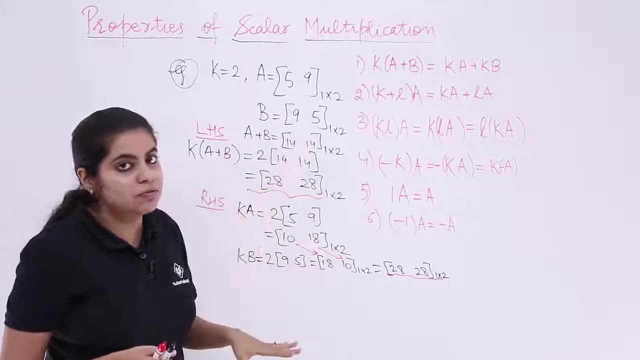 means LHS and RHS is same. and when LHS and RHS is same, the first thing, we have already proved so in this manner, you can prove it with the help of examples. now, after the first part is done for the properties, let's move on to the second property. the second property. 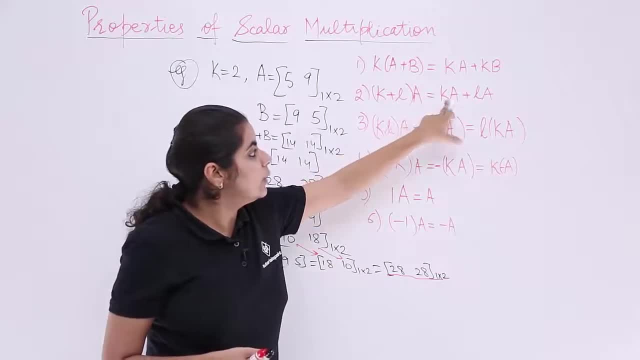 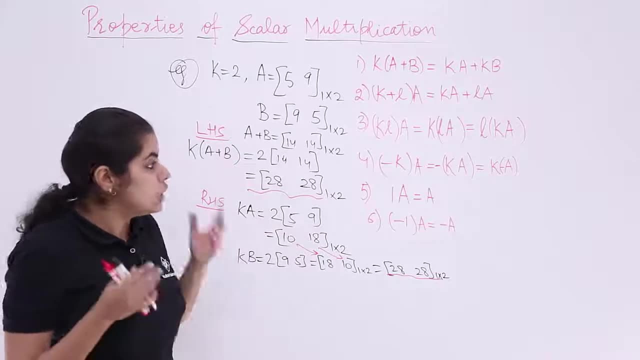 is what it is: K plus L into A is equal to Ka plus La. that means this time we don't have two matrices, we have only one matrix and we have two scalars. so let's start with this proof, also with the help of example. I will be rubbing the board from this part and now. 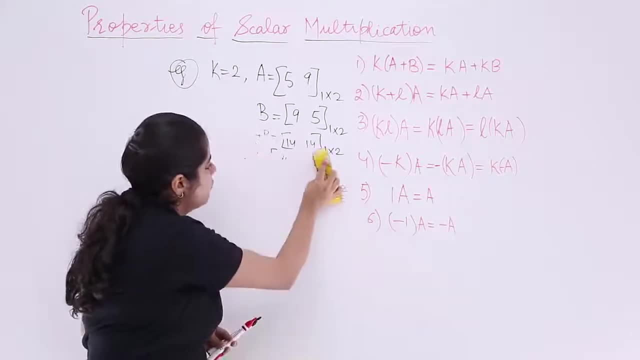 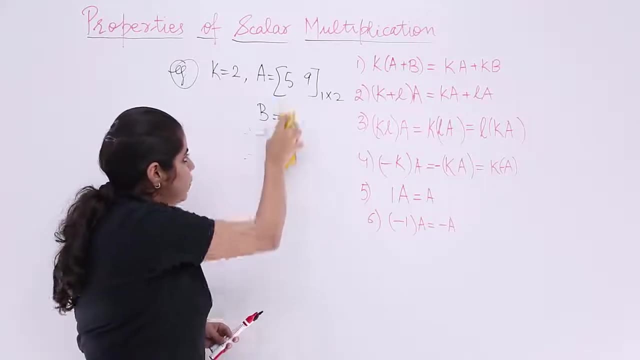 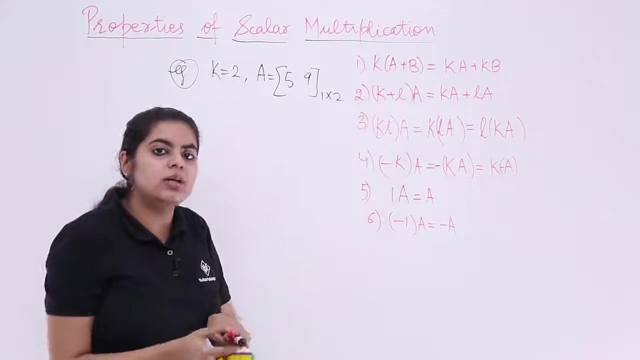 we will be doing it in this video. we have many parts, and we will be taking the proof in the form of properties with the help of few examples, right? so, since I don't need only K, we need L also, let's take another scalar quantity, with the help of which we will be. 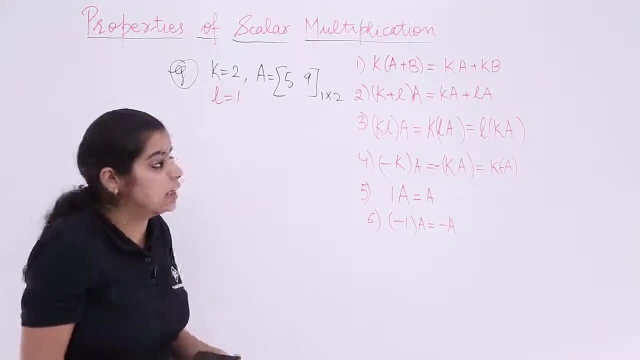 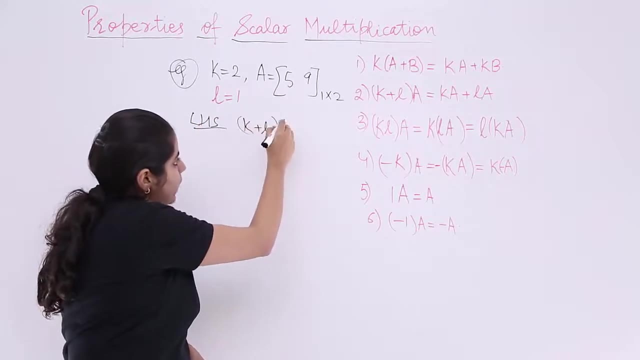 solving it. let L be 1, any value that you can take Right. so the left hand side is K plus L- into A. I put the heading LHS- it is K plus L- into A. now what is K plus L? K plus L is given to me as 2 plus 1. what is 2 plus 1? 2 plus 1 is. 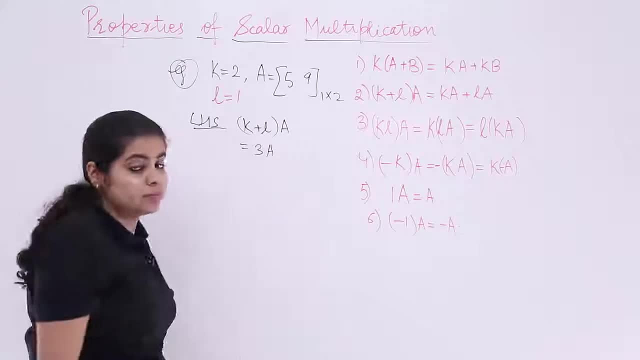 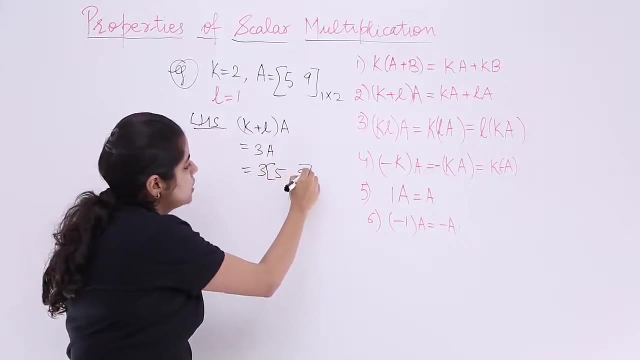 3, right, so it is 3 into A. that means what you need to multiply the matrix A by 3, so it is 3 into the matrix A, which is 5- 9. now, what is 3? 5s are 15. what is 3: 9s are 27. so 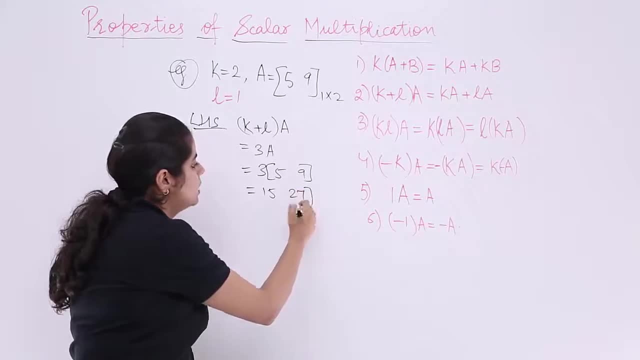 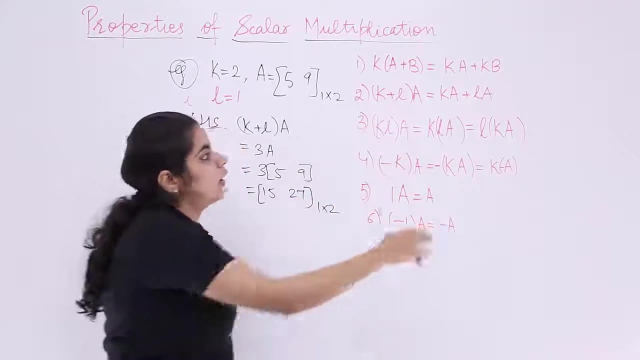 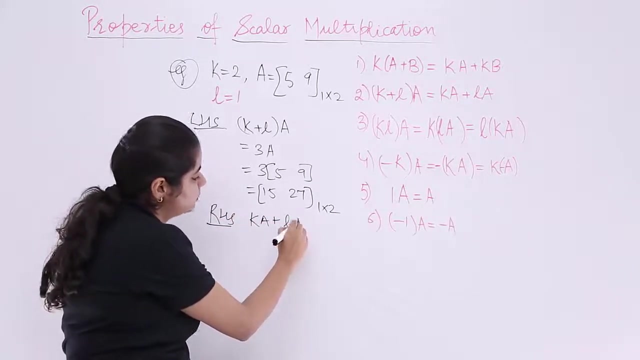 it is 15.. 15 and 27. that should be here in this matrix and it is a 1 by 2 matrix. this is done as per the first part, LHS. what about the right hand side? right hand side, quickly, let's do it. RHS is KA plus LA. what is the value of K? K, we know, is 2. K into A means 2 into A. 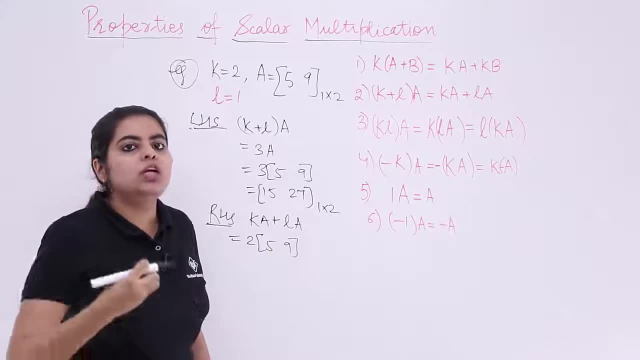 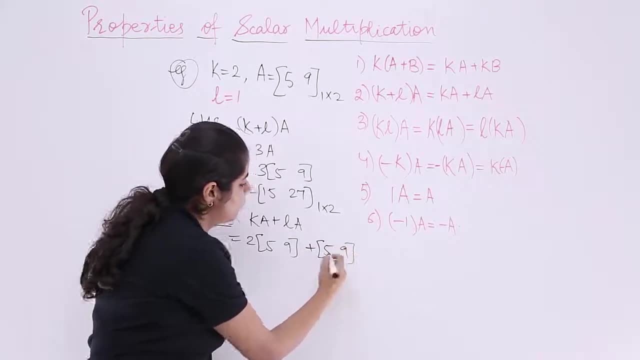 plus L into A. what is L? L is 1, 1 into 2.. 2, 1 into 5, 5. so 1 into the matrix is the same matrix, no change. now what is 2, 5s are? 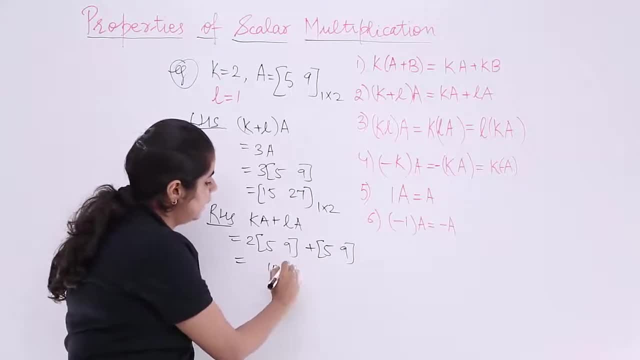 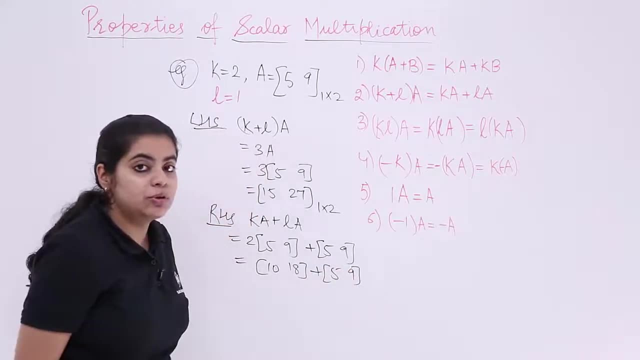 it is 10, 2 9s are is 18. so 10 and 18 are the elements here. what about the other side? it is 5 and 9. now you need to add them. what is 10 plus 5? that is 15. what is 18 plus 9 that? 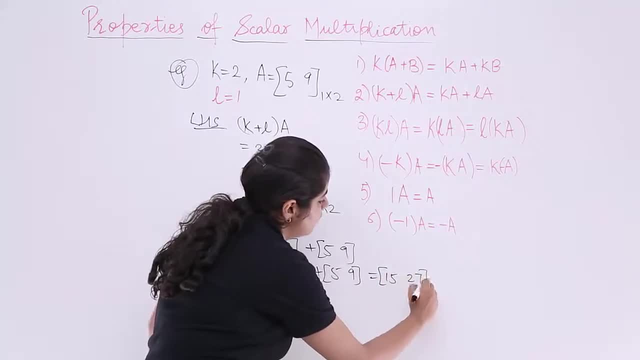 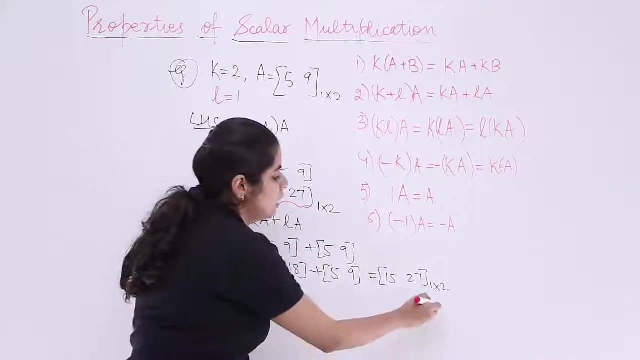 is 27, so I basically get 15 and 27 1 by 2.. So this is the matrix. So this is the matrix. So this is the matrix. Now see what was the answer earlier: 15 and 27. what answer now? 15 and 27. that means both. 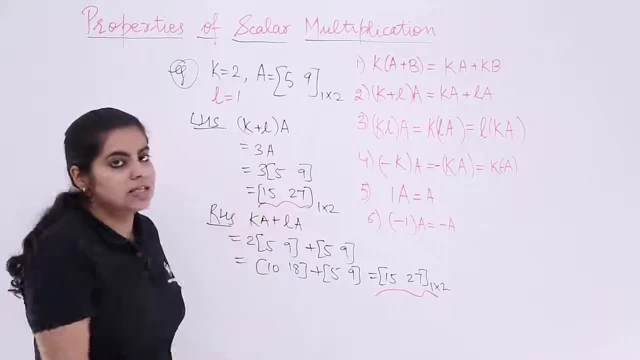 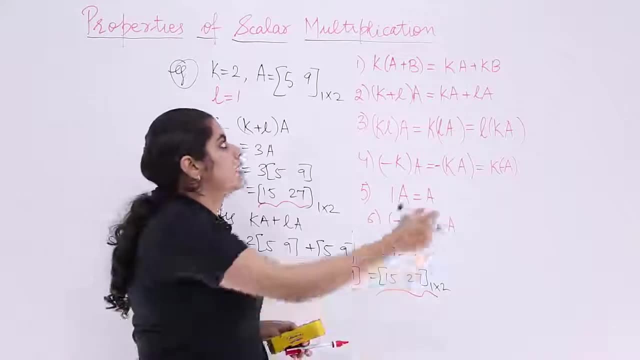 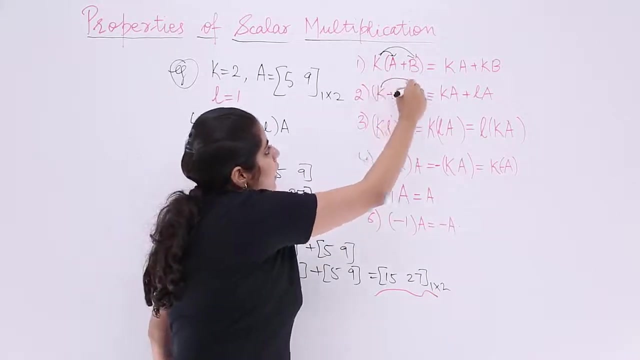 these values are same and that means LHS and RHS are same. so that means we have proved K plus L into A is equal to KA plus LA. one thing that I need to show again and again is it is simply the distribution: K into A plus K into B. here also, K into A plus L into. 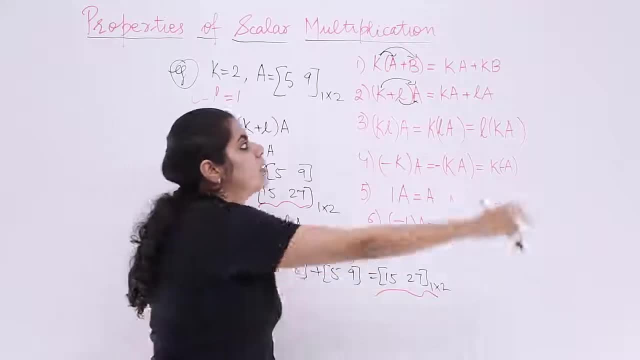 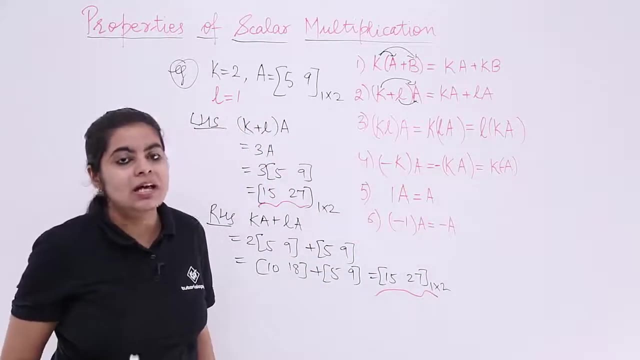 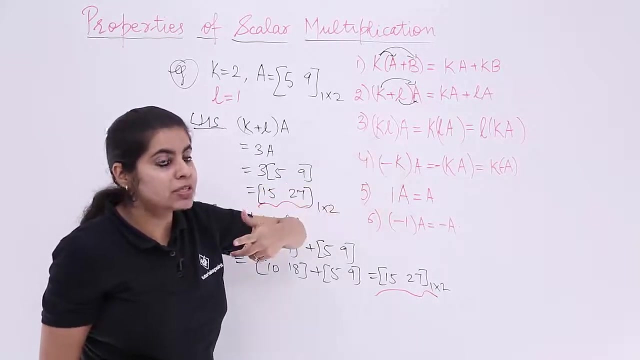 A, the only difference between the first and the second property. The first property had two matrices, one scalar. second property has two scalars, one matrix. now, when we have understood these two, let's move on to the third one. the third has two scalars again, but the difference is what? earlier it was addition, this time it is multiplication. 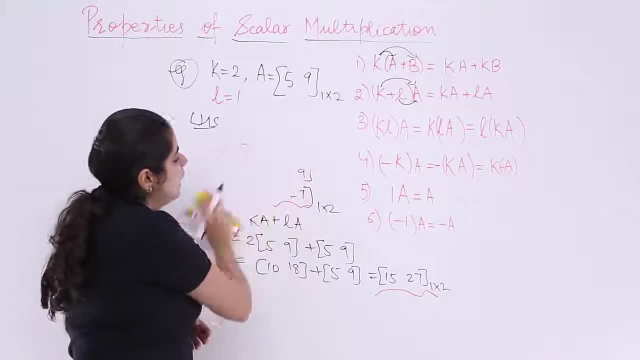 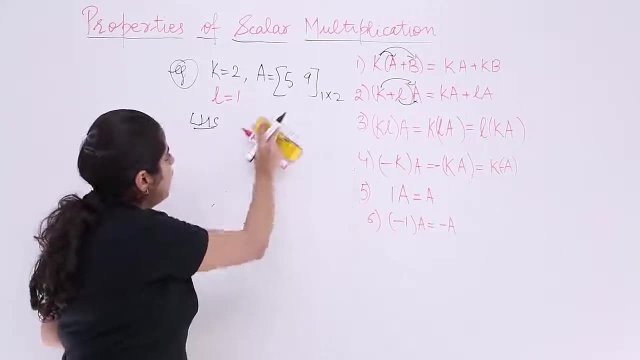 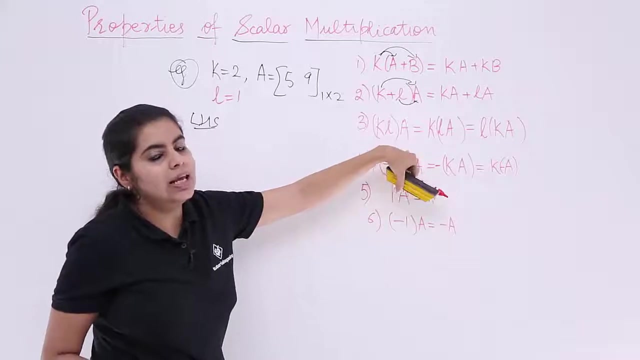 similar things, similar steps. quickly, let's do it. we will be taking LHS, we will be taking RHS, we will be proving the values and we will be getting the answer. A very quick answer And fast way to do it in the form of proof. LHS, KLA, K into L, two ones are, is what two? so 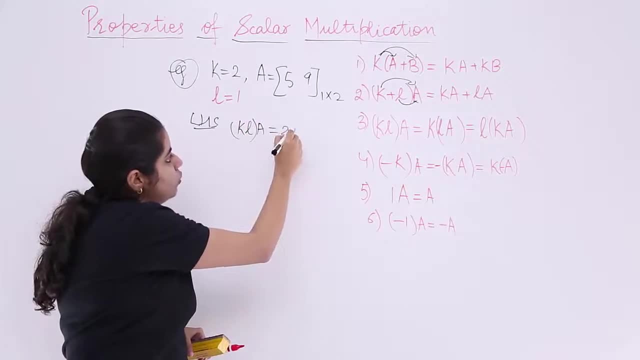 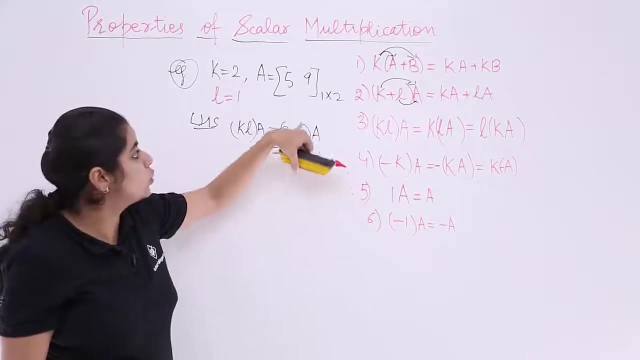 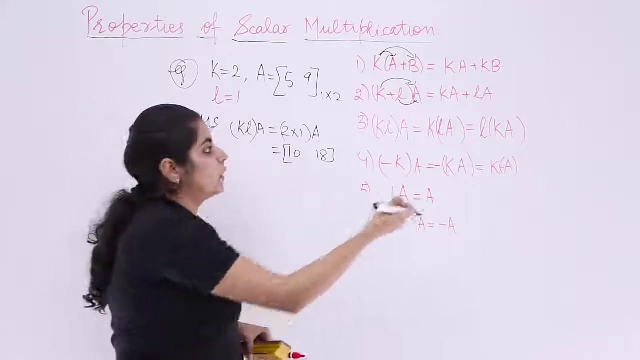 KLA, that means two multiply by one. multiply by A, that means two ones are two and two into A matrix. so two into A matrix is two. fives are 10, two nines are 18. so that is LHS, that is done. What about the second case? 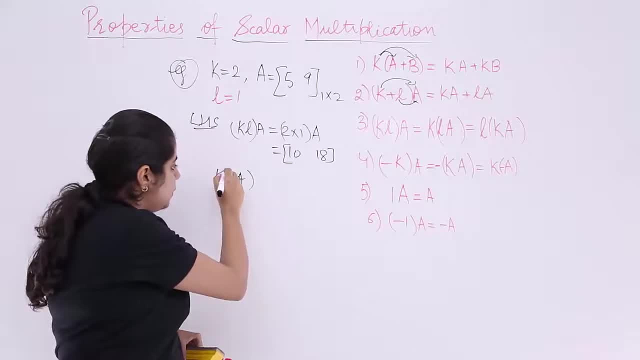 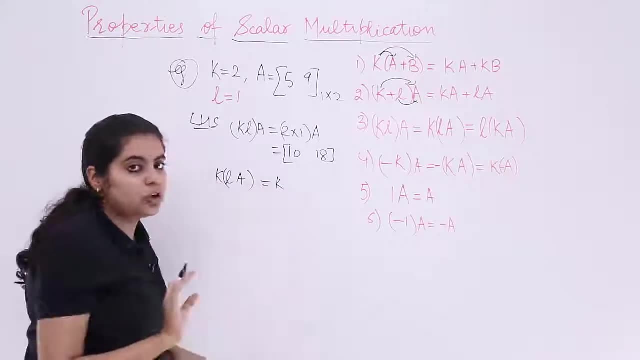 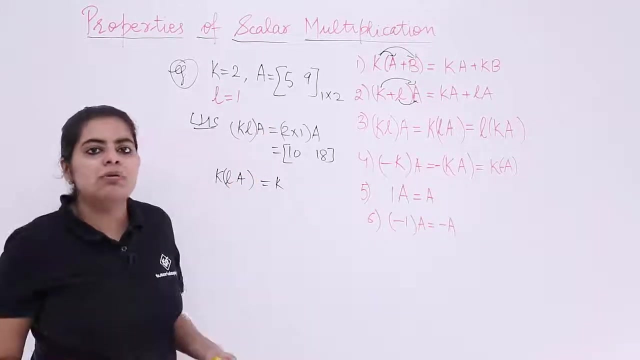 What about the second case? Second case is again KLA. but first we need to do what we need to solve L and A. let's do it. K outside, only K need not be changed. L into A, L is what L is: a scalar. that scalar has the value as one, so one into a matrix does not change it. that means we have the. 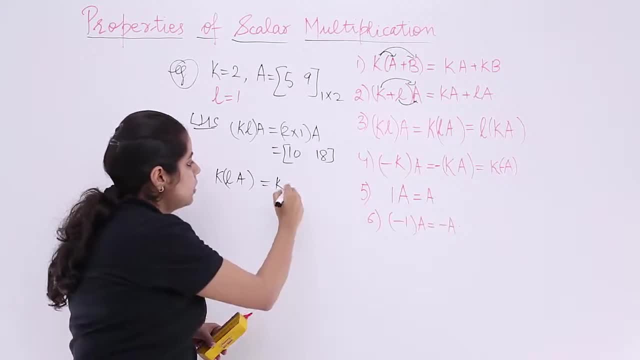 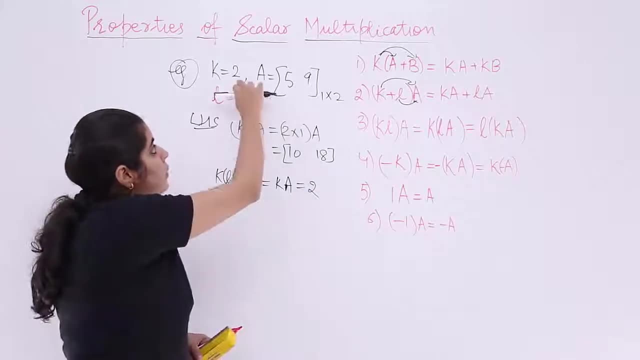 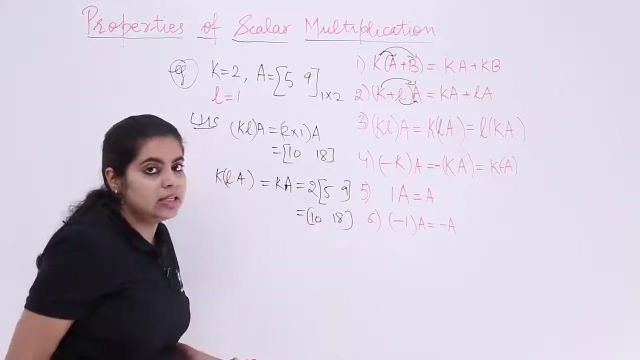 matrix only, which is A. no change in the matrix K into A. K is what it is. two. you see here, from where, from the above, what about A? again, it is five and nine. two fives are is 10, two nines are is 18, 10 and 18. last but not the least, LKA. LKA means what? let's see where the 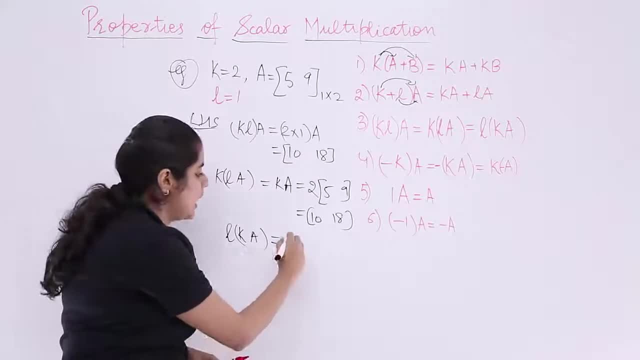 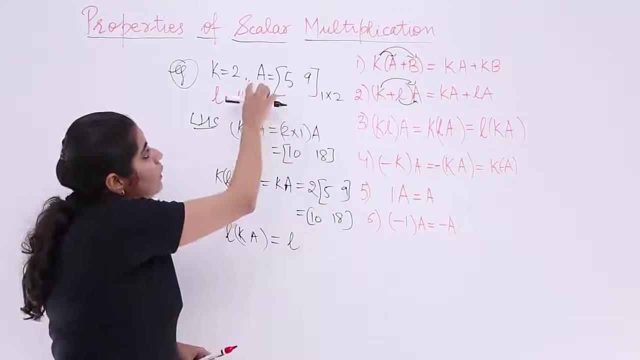 brackets are there. you need to solve them first. K and A are there L outside only. K is two and A is a matrix. so two into the matrix. what is the result of two into the matrix? two fives are 10, two nines are 18.. 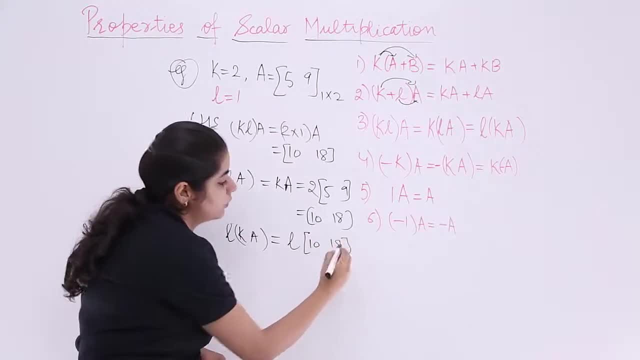 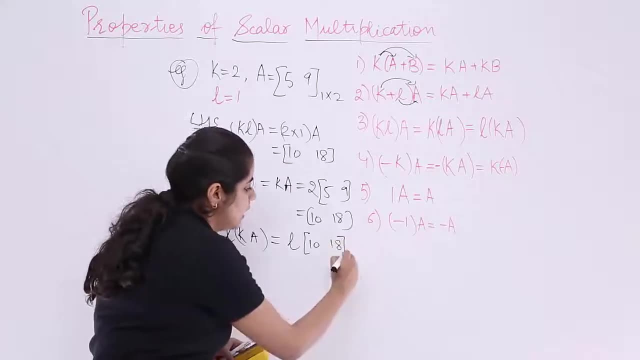 So it is two and A is a matrix. so two into the matrix. what is the result of two into the matrix? So what is 10? and 18 put the value of L. what is L? L we had taken as one. so that means what that means. basically, I need to multiply the matrix by one, multiplying the matrix by one. 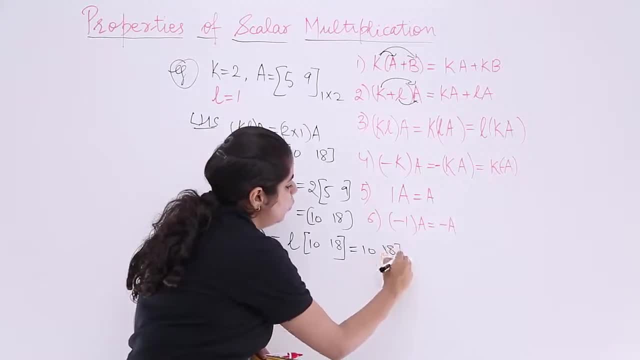 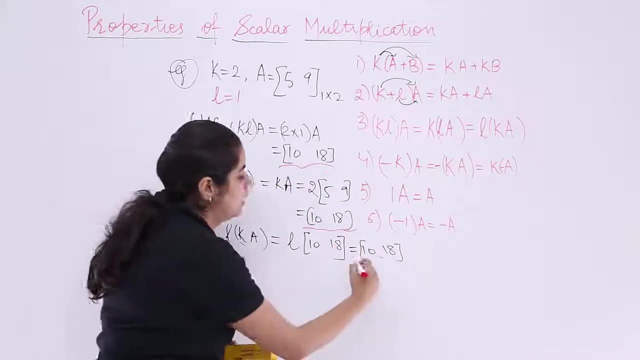 does not change the answer. so it is 10 and 18. only now compare the answers. comparing here it is 10- 18. next case: 10, 18 again, the next case: 10, 18 again. the three cases have the same answer. that means this property is proved. how to learn this? 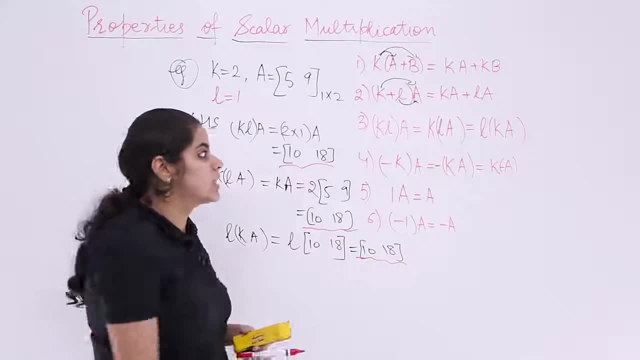 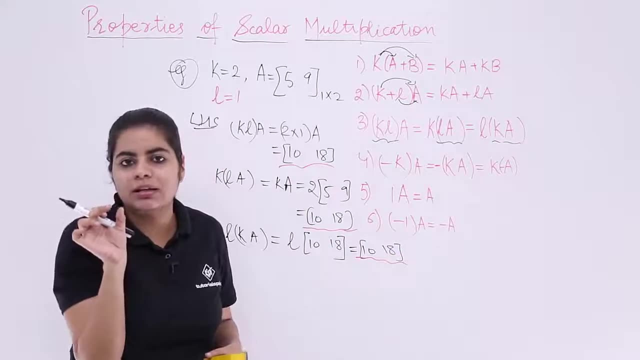 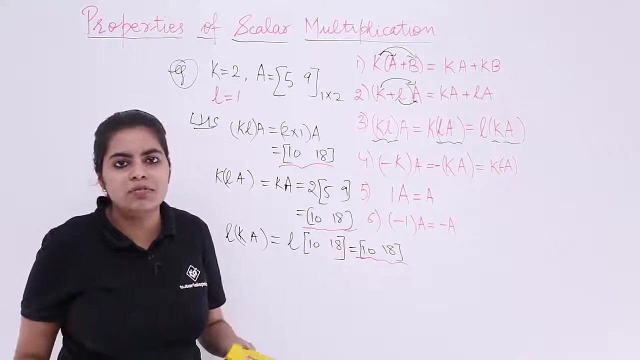 I have two scalars. one, multiplication value of matrix. firstly, bracket on the first two, then bracket on the last two, and then I mean taking any two things at a time. the other, keeping it aside, does not change the answer. you do whatever for the matrices, multiply whatever first, lastly, anything, the answer does not change. so in this case we proved. 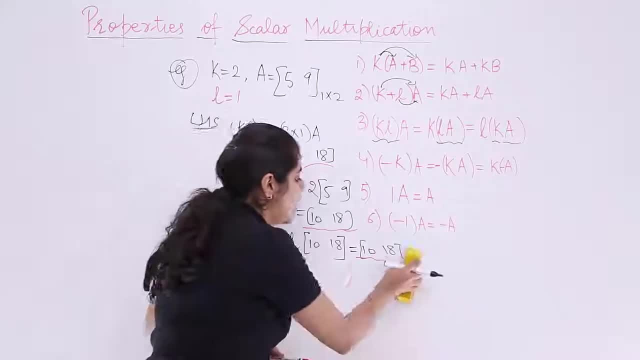 the third property as well. let's move quickly to the fourth one. I will be raising this board for the convenience. 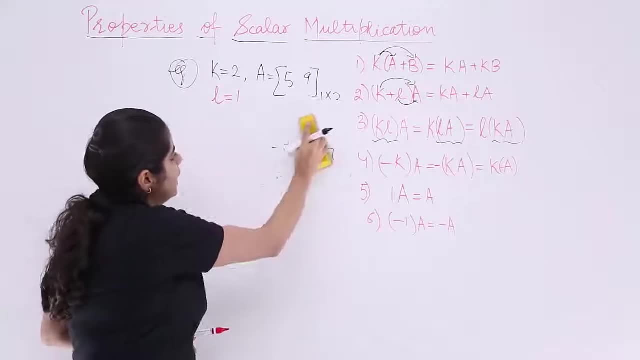 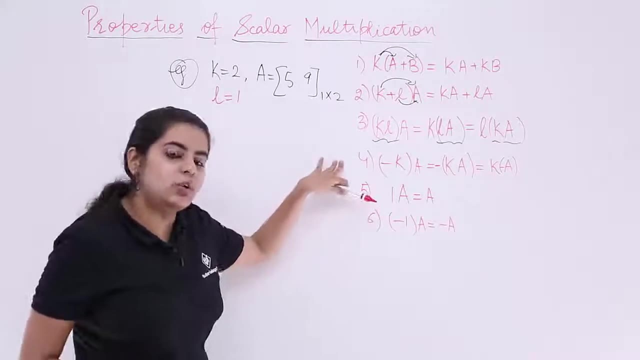 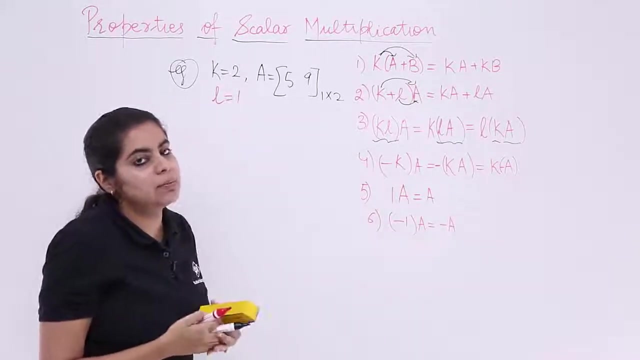 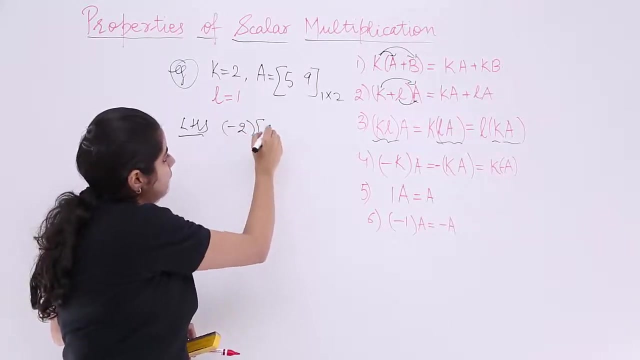 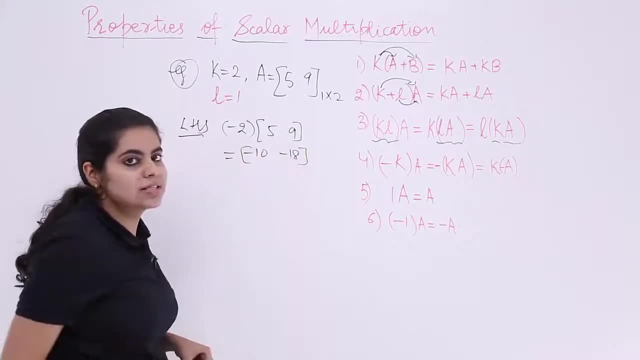 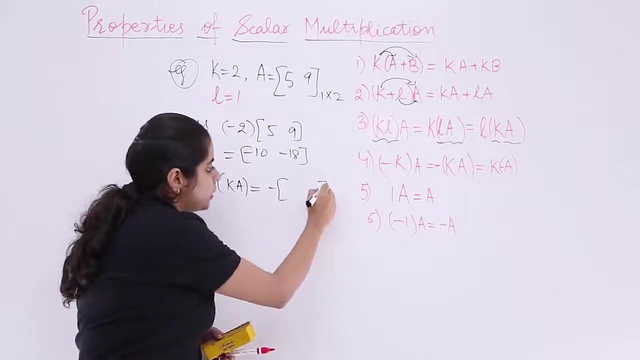 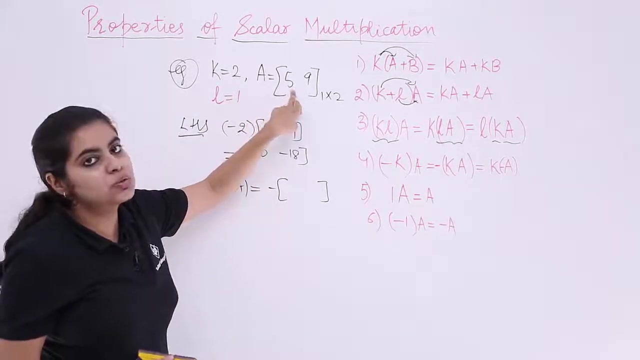 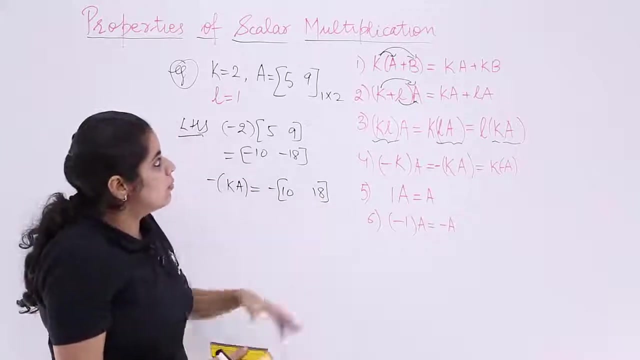 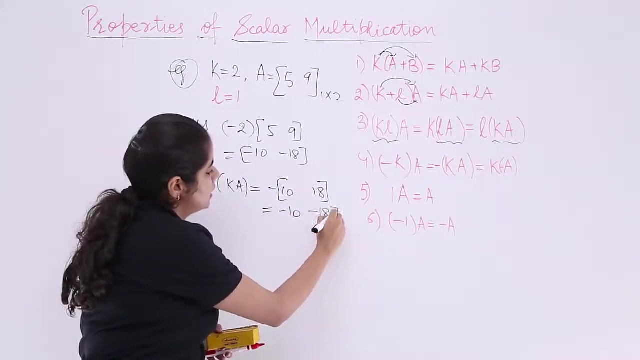 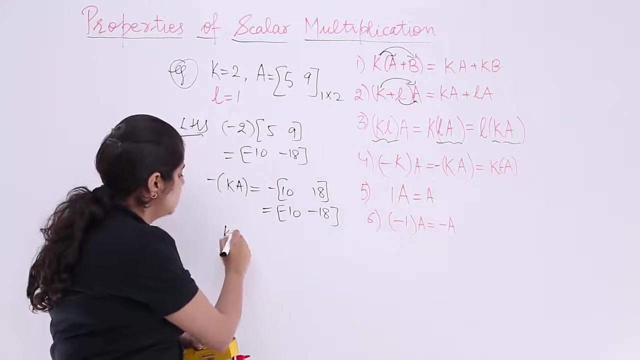 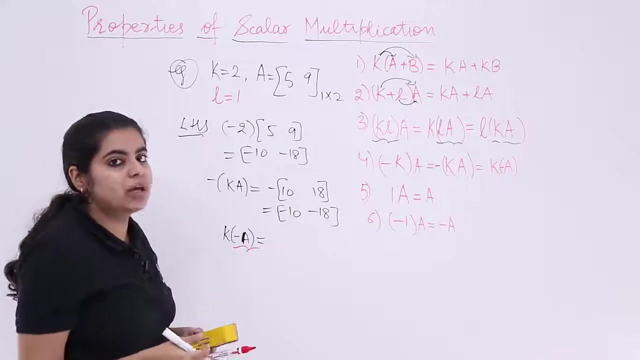 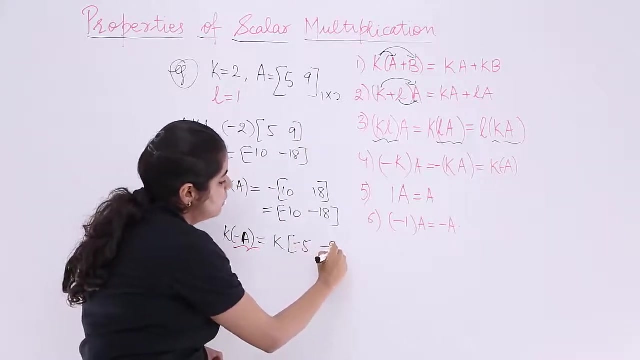 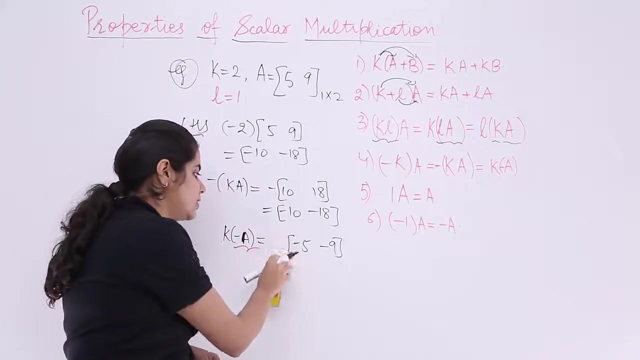 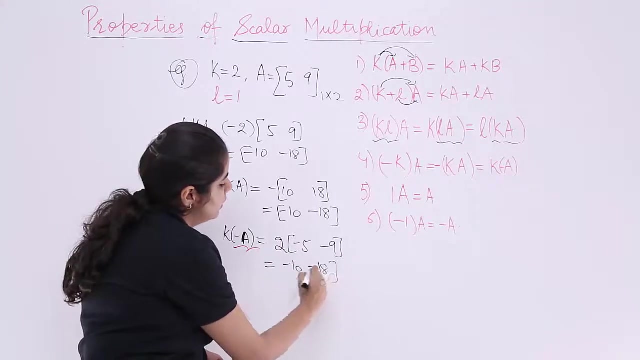 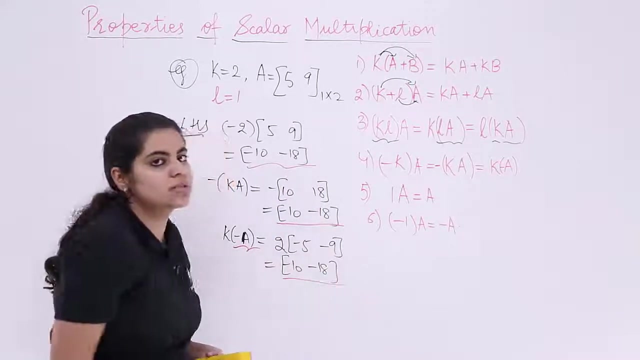 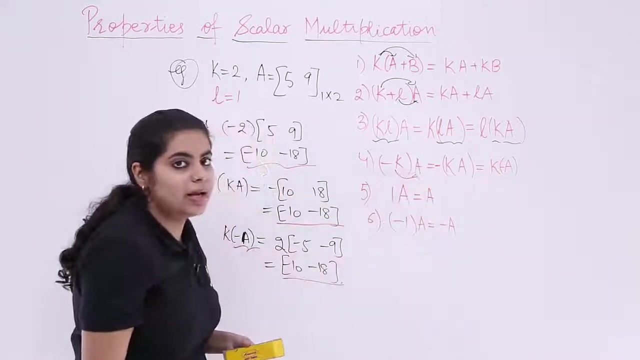 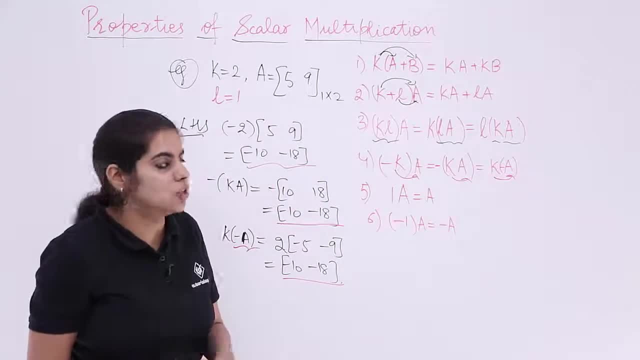 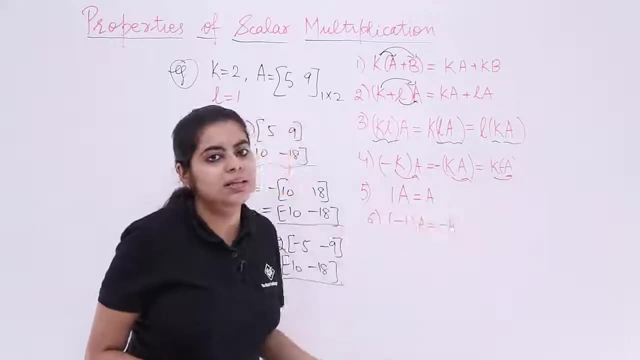 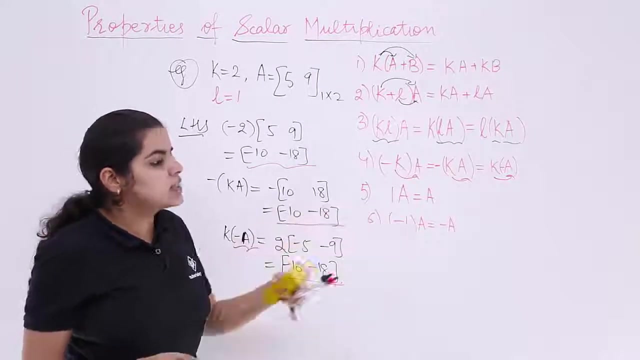 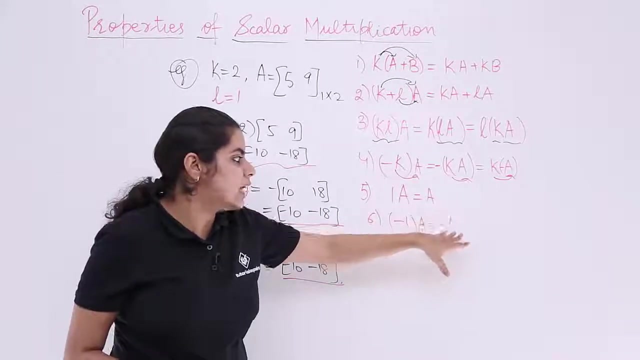